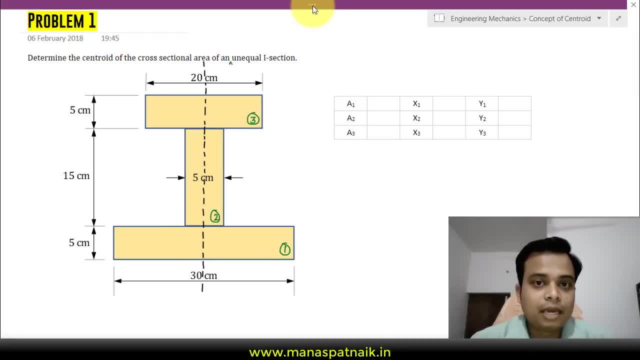 eventually. okay, fine, now let's go ahead, and first of all, let me have the coordinate axis. that will be better. um, it's, it's something like this: yeah, pretty good, and now let me let me fit this in properly. yeah, let me write: this is the y-axis and this over here represents the x-axis. so what we wish to do, 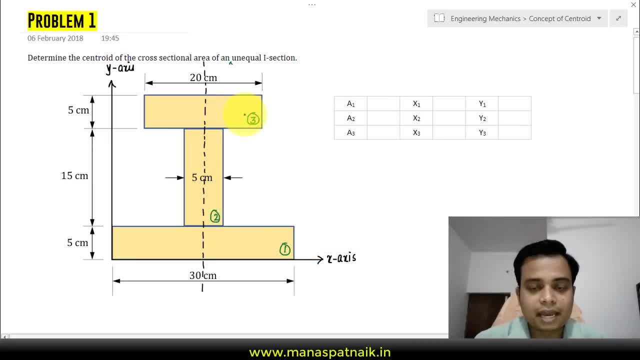 is we need to fail this table corresponding to these three rectangles. we have the values of their areas, their corresponding x coordinates and their corresponding y coordinates. let's kick off by calculating the areas. so, first of all, we have this rectangle. this: its area is going to be: 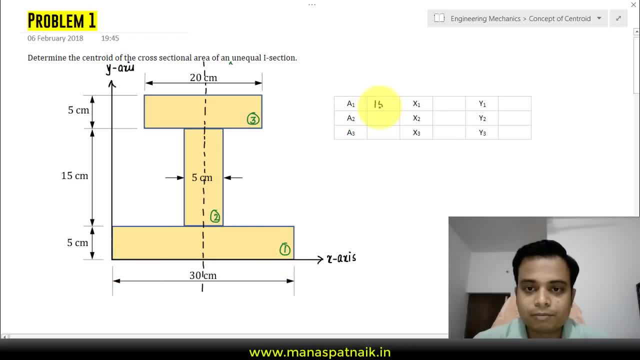 30 multiplied by 5 and that's 150.. pretty simple. secondly, we have this area um, this is how much that's 5 and this is how much that's 15 for 5 cross 15 is 75, pretty simple. and then, finally, we have this: 20 cross 5 and that's 100.. so you have to. if you sum them up, the total. 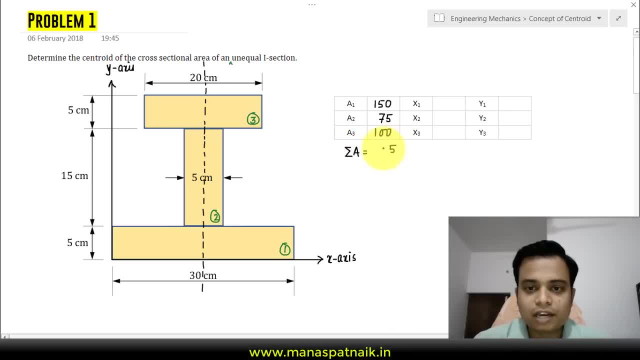 area that we're going to work out is going to be equal to. this is 5. 7 plus 5 is 12. carry 1, that's 3 325 centimeter square, obviously. well, this calculation will be done in centimeters. this will also be done in centimeters. now let's go ahead. 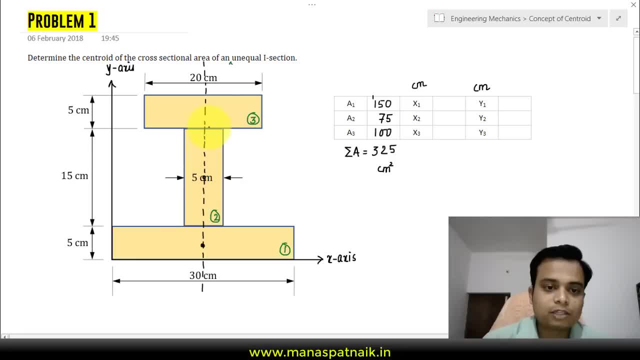 and let's calculate the value of x1. okay, this is going to be x2 and this is going to be x3. now guys watch carefully this: this essentially represents the value of x1. okay, that's x1. this represents x2, x2 and this represents x3. what's common in all of these? their lengths are common. 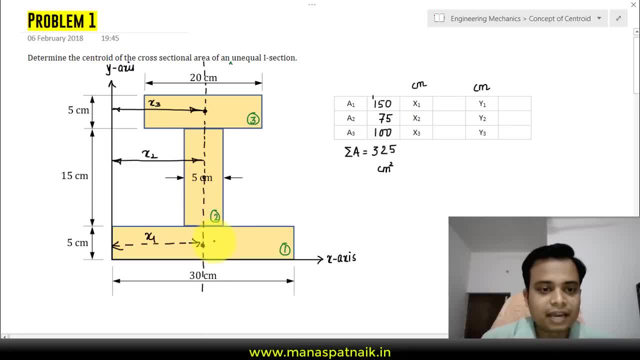 so since the centroid of all the individual rectangles are lying on this vertical line, therefore their x coordinates are going to be same and all of them are going to be equal to 15. let me tell you that. okay. so this is how much. that's 30. so half of 30 is going to be 15.. so x1 will be 15. 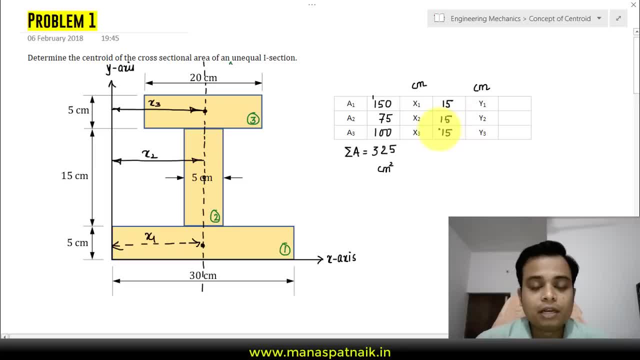 x2 will be 15 and x3 also will be 15.. now we only need to worry about their y coordinates. okay, now you can say that their individual centroids are represented by c1, c2 and c3. right now, let me have a, let me have a red color. this over here, this small distance that you guys see is what you refer to as. 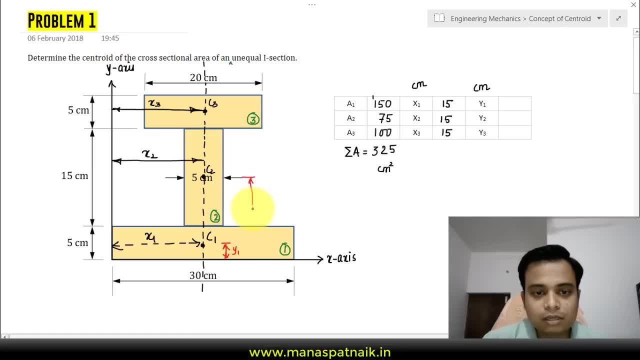 y1. okay, this distance over here that you see, that is y2, and this distance over here, okay, that's y3. extremely sorry, I cannot draw a straight line with you. the help of this pen tablet. okay. so how much is y1? this is how much in totality from here till we. 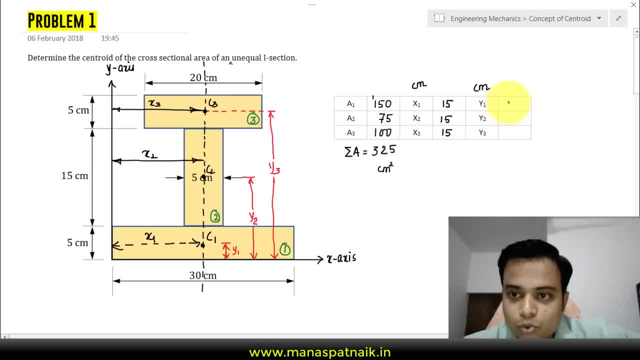 reach here. that's 5, so half of 5 is 2.5. so y1 is nothing but 2.5. pretty simple, straightforward, okay. so in order to get the value of y2, you need this distance, okay, and you can clearly see from. 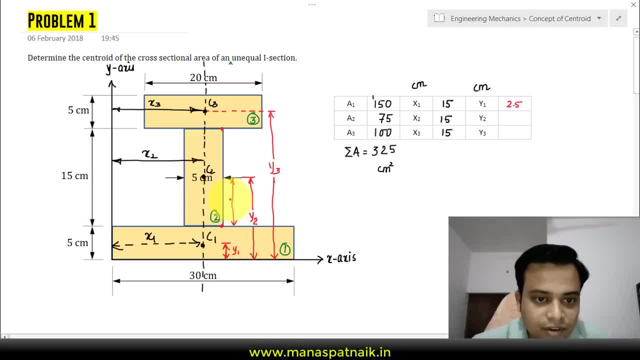 here to here this: that distance is how much 15. so half of 15 is 7.5, so that's 7.5. so in order to get the value of y2, we have this much: from here to here, that's 5, plus from here to here, that's 5, 5 plus 7.5 is 12.5. that's 12.5. 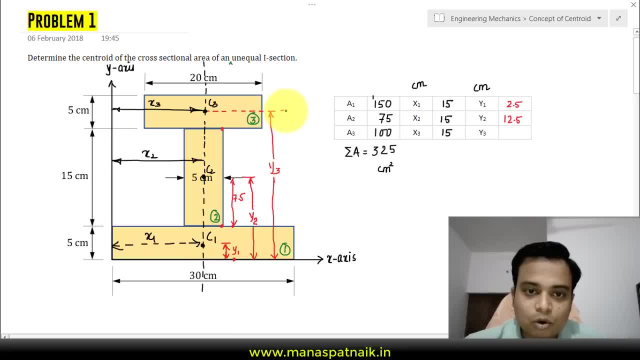 done, and then, finally, we have to find the value of y3, and that's also pretty simple. how much is this, tell me. that's half of 5, that's 2.5. so you need to add this length from here to here to this 2.5. then you can finally have the value of y3. this is going to be fairly simple. 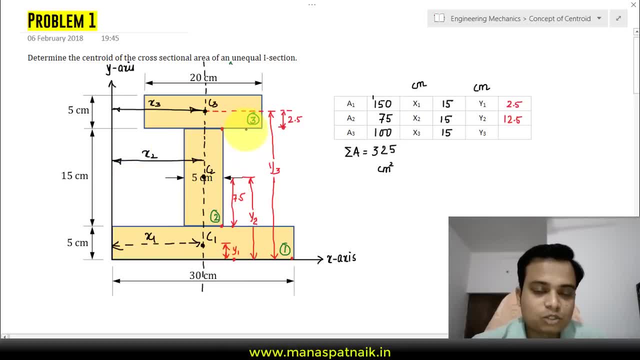 um, this is 5. 5 plus 15 is 20. 20 plus 2.5 is nothing but 22.5. okay, so that is essentially done. now now? now, what can we do? well, we have this final formula in order to calculate the value of centroid. okay, it's something like this: it's a1- x1 plus a2 x2.